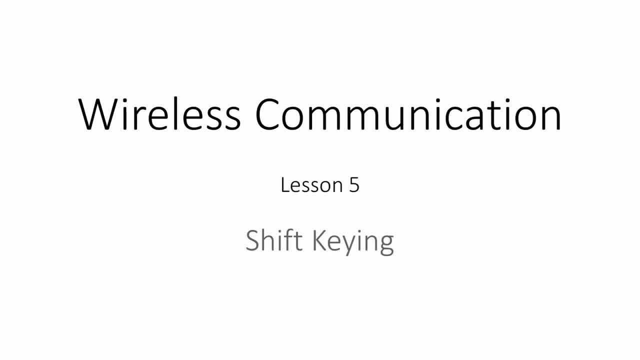 In this lesson, you'll learn about shift keying. Shift keying is the term used for the modulation of digital data. There are four main types of keying: On-off keying, amplitude shift keying, frequency shift keying and phase shift keying. Let's take a look at each. 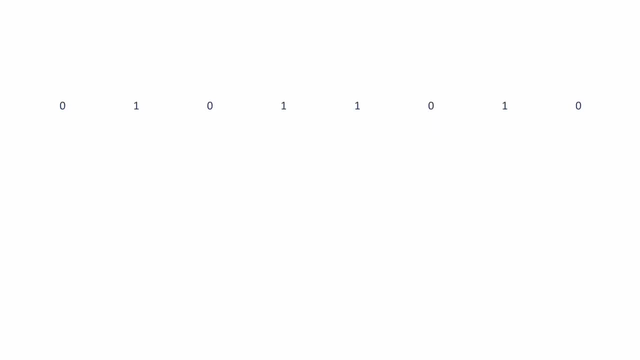 These days, most of the data we communicate wirelessly start off as digital data: a stream of binary 1's and 0's Inside a computer. binary digits are represented by electrical pulses which, when shown on a graph of voltage against time. 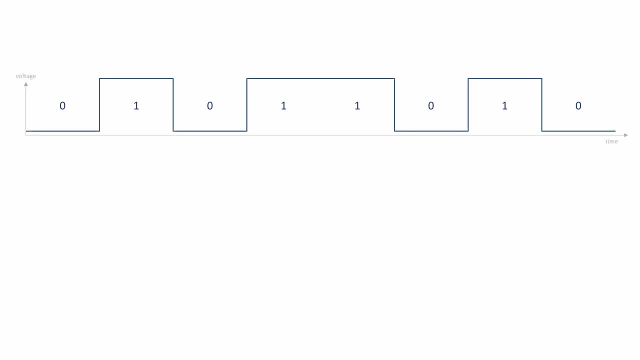 result in this familiar square wave visualisation that most students of computer science would recognise. When the voltage is relatively high, it can be seen in a singular direction, as shown here. If the energy in a digital pulse is equal, then it can be proven from the operation. 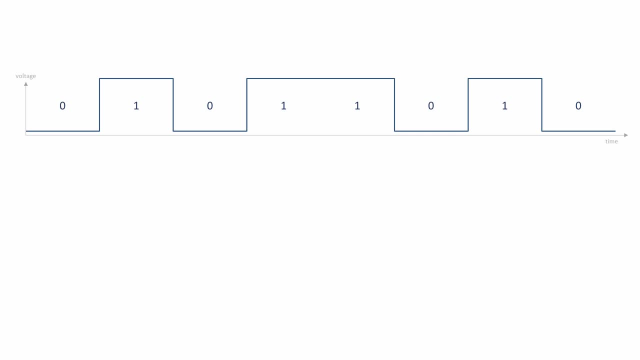 high, we have a 1.. When it's low, we have a 0.. Each of these two possible states is known as a symbol, and a stream of symbols is referred to as the baseband signal. Before the baseband signal can be transmitted via radio, it must be modulated. It needs. 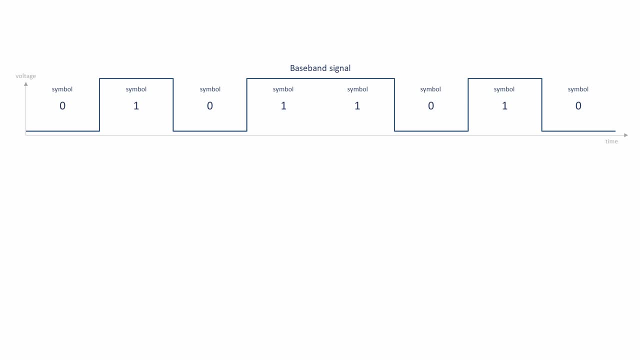 to be converted into a form that can be radiated by an antenna. It also has to fall within a particular frequency range in order to comply with the law. The simplest way to achieve this is with on-off keying, or OOK for short. This involves a 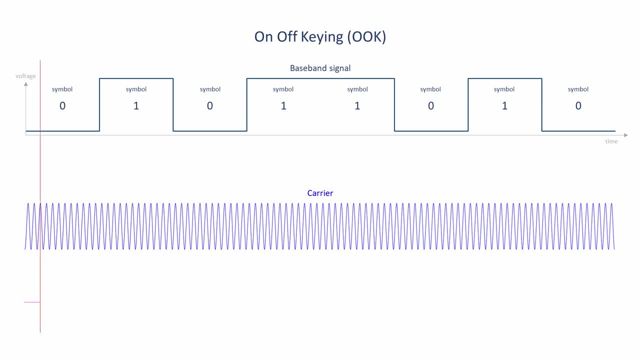 continuous wave carrier which is generated within the transmitter. Then, one symbol at a time, the data are encoded on the carrier by simply turning it on and off with little more than a switch, rather like Marconi did in 1897.. Another way to encode binary data on the carrier wave is with Amplitude Shift Keying. 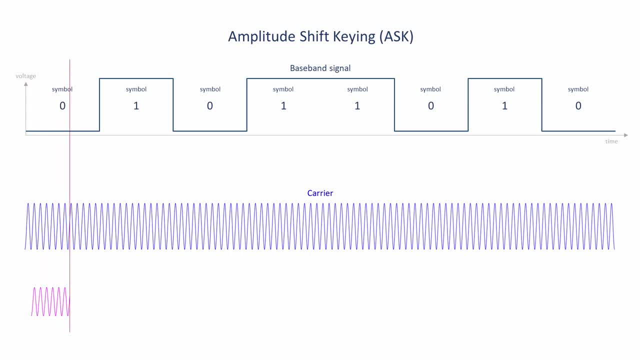 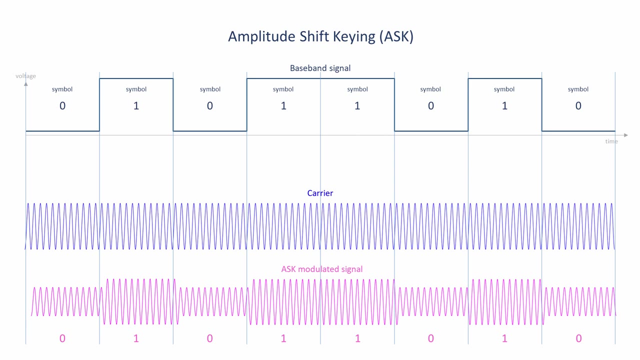 or ASK for short. With amplitude shift keying, the digital signal is multiplied by the carrier. Whenever there is a drop in the voltage of the digital signal, which never quite falls to zero, there is a drop in the amplitude of the carrier. 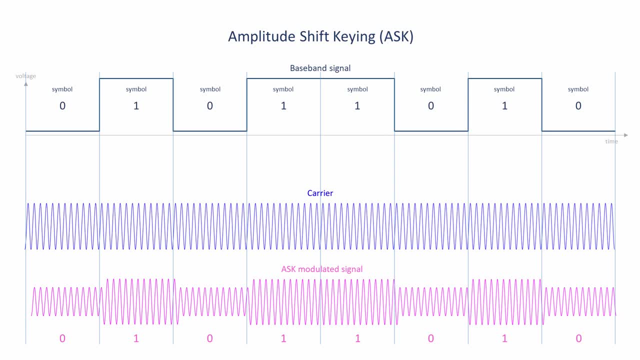 When the voltage drops, the signal is actually multiplied by the current- I'm going to change- of the digital signal increases, so does the amplitude of the carrier, As, with on-off keying, the modulated signal is now in one of only two possible states. 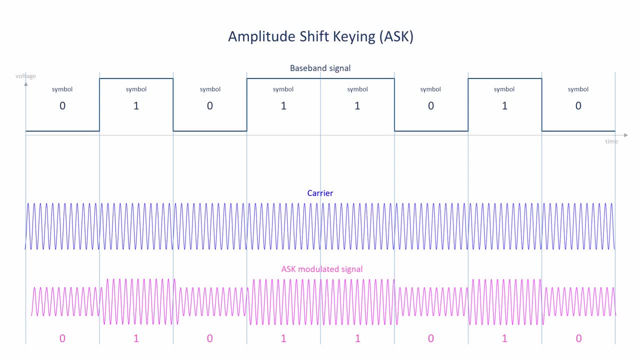 When the amplitude of the signal is relatively high, it's carrying a 1.. When it's relatively low, it's carrying a 0.. The rate at which the modulated signal changes from one state to another is the same as the symbol rate. 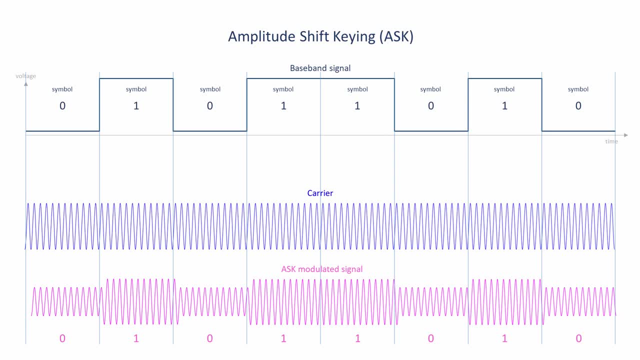 One after another, each waveform is converted into radio energy by the antenna, and it's propagated through space. At the receiving end, the incoming signal is sampled at the symbol rate, and the amplitude of each sample is used to determine whether it represents a 1 or a 0. 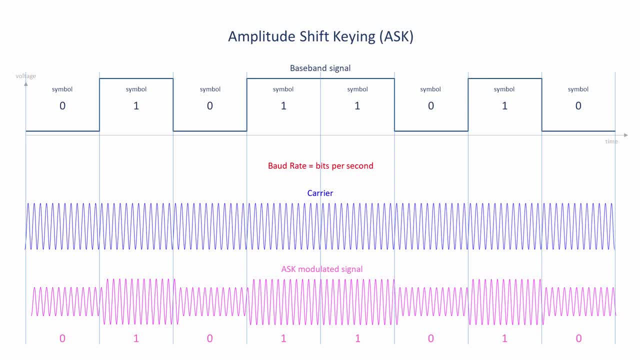 The number of bits transmitted per second is known as the board rate, The simple implementation of amplitude shift keying that you can see here. The principle of amplitude shift keying can be taken a stage further. Rather than only two possible waveforms in the modulated signal, there could be four. 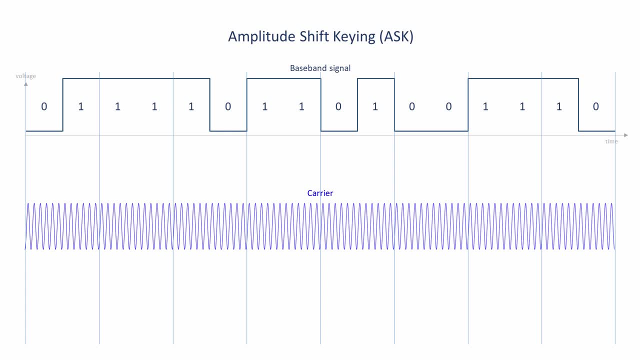 each with a different amplitude. Each waveform could represent a combination of two bits. With two bits per symbol, the board rate would be doubled, so twice the amplitude has been repeated. Now let's make a simple equation. Let's say that the amplitude of the signal on the Y-axis is 0.. 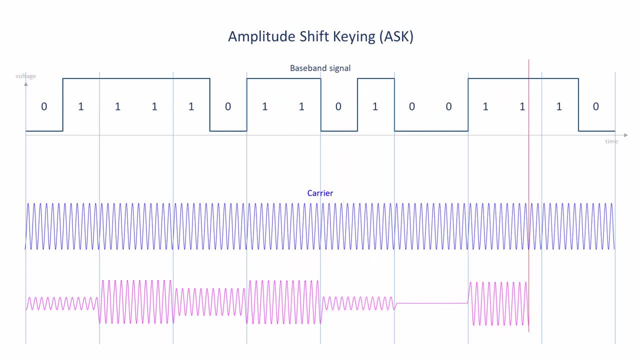 So twice as much data could be transmitted in the same amount of time. Theoretically, there could be even more waveforms in the modulated signal, each with a different amplitude. Eight possible amplitudes, for example, would allow the transmission of three bits at once. 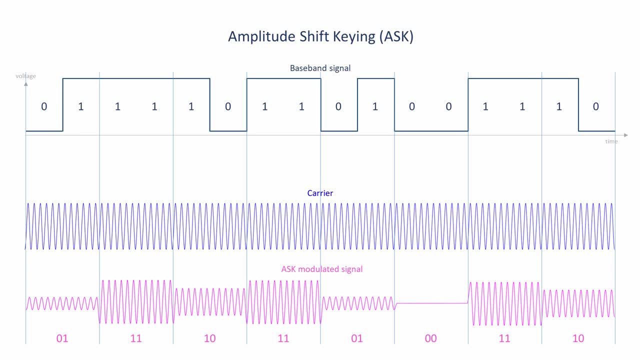 There is, however, a downside to scaling up the baud rate like this. The receiver has to be able to distinguish one waveform from another, and the more of them there are, the closer their amplitudes will be. Amplitude shift keying is already susceptible to amplitude variations due to external interference. 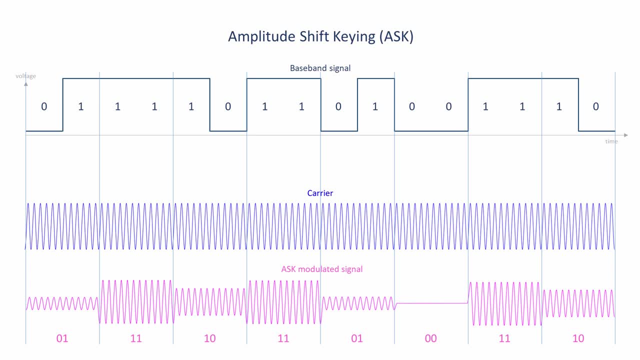 so a high baud rate could make matters much worse. Nevertheless, ASK and OOK are commonly used in short-range wireless applications in the home to control things such as lighting, heating and kitchen appliances. ASK is also used to transmit digital data. 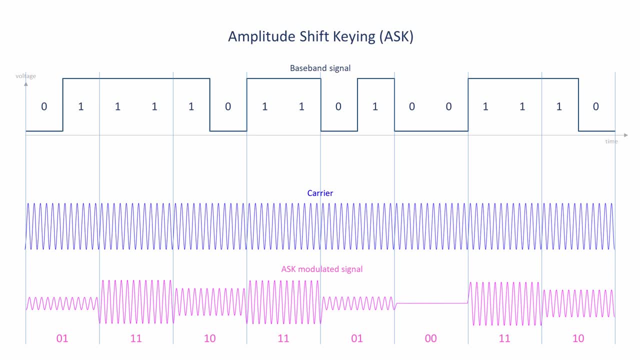 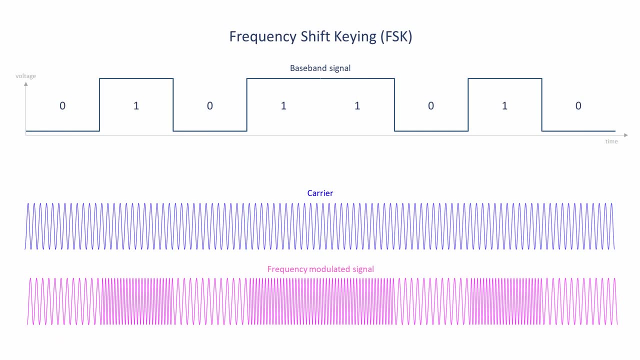 An alternative way to communicate digital data via radio is with frequency shift keying. As with amplitude shift keying, a continuous wave carrier is generated and modified according to the digital signal. But with frequency shift keying, a 1 is represented by a relatively high frequency in the modulated. 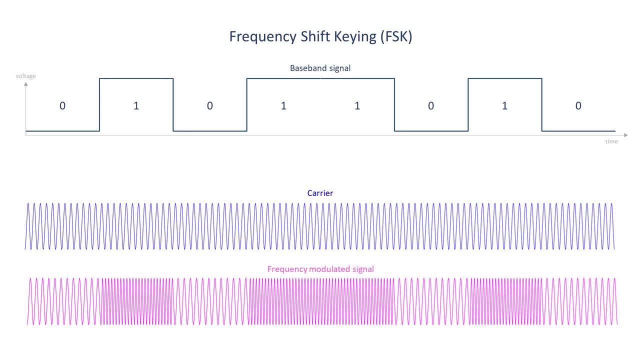 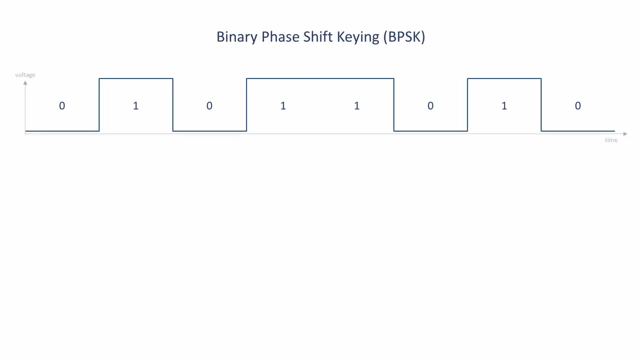 wave A 0 is represented by a lower frequency. Frequency shift keying is less susceptible to interference, because interference tends to affect amplitude rather than frequency. The obvious downside, however, is the increased bandwidth of an FSK signal, Perhaps the most important development in the communication of digital data via radio. 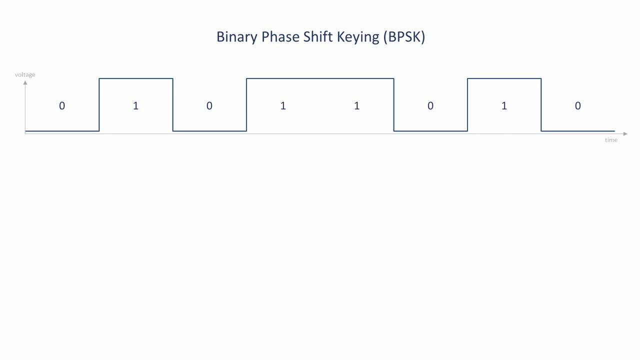 has been phase shift keying, also known as binary phase shift keying, or BPSK for short. Before the carrier is modulated, the baseband signal is modified such that a 1 is now represented by a positive voltage and a 0 is represented by a negative voltage. 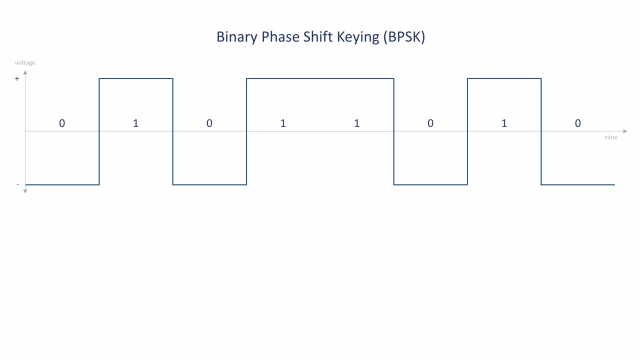 Preparing the baseband signal like this is called line coding, and there are various ways it can be done, as you'll see later. This particular line coding scheme has resulted in what is known as a polar non-return to 0, baseband signal. 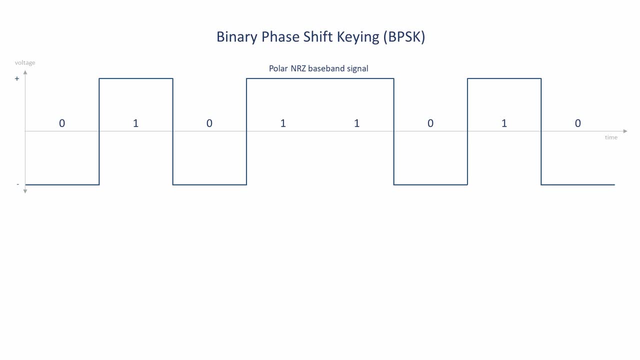 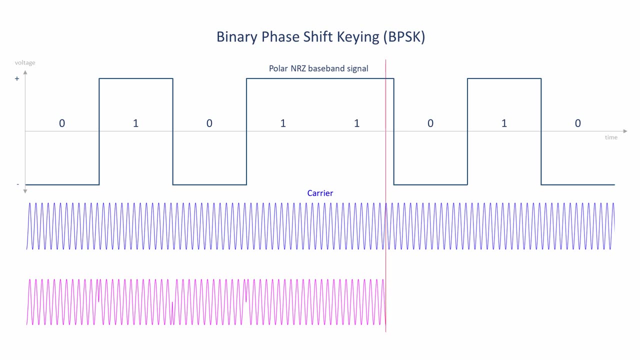 One symbol after another. the square wave is multiplied by the carrier, as is the case with amplitude modulation, But because the modulating signal is an NRZ signal, the carrier is inverted whenever there's a change to zero or zero to one. This is effectively a phase change, A swing from. 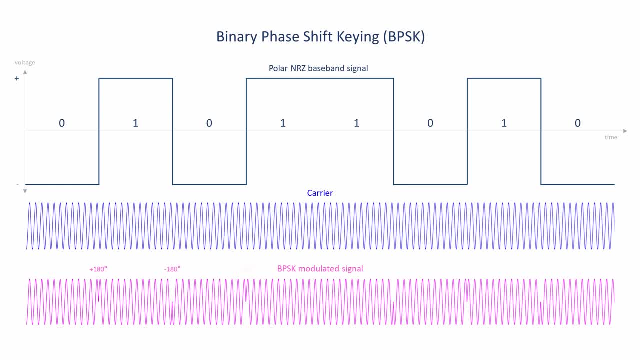 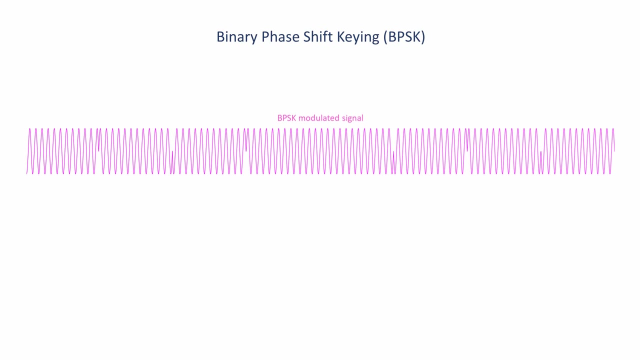 zero to one in the baseband signal results in a positive phase shift in the carrier of 180 degrees, and the swing from one to zero results in a negative phase shift of 180 degrees. At the receiver, the modulated wave is converted back into binary digits. The receiver does this by comparing the